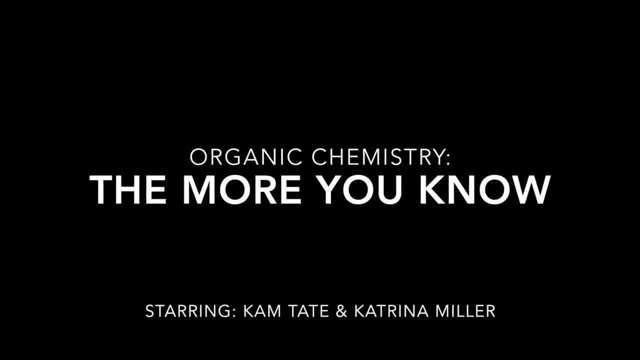 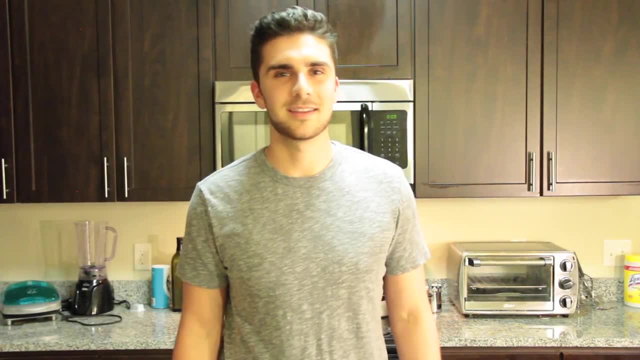 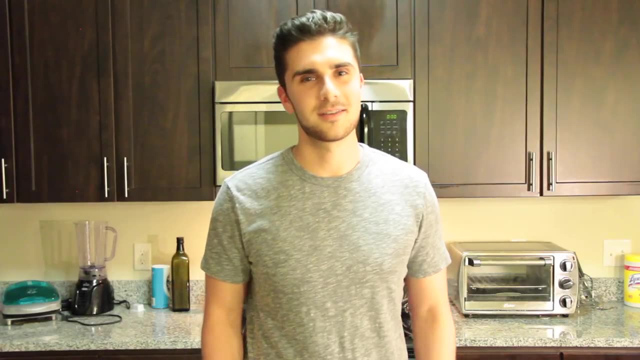 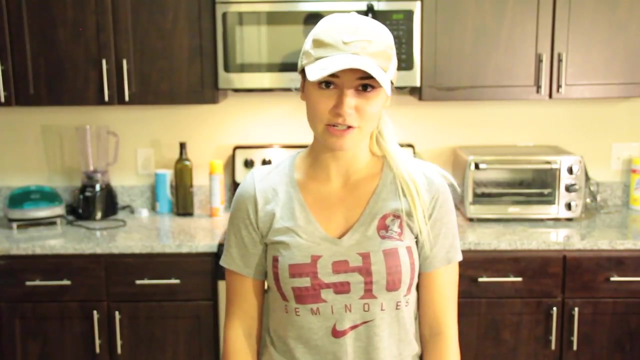 Oh, it's you. I know you're thinking organic chemistry is hard as ****, but I'm here to make it a little bit easier with some real world applications for the chemistry we call organic. Organic chemistry is involved in everything around us: Cooking, cleaning and even the gas that runs your cars. But today we're going to keep it in the kitchen. 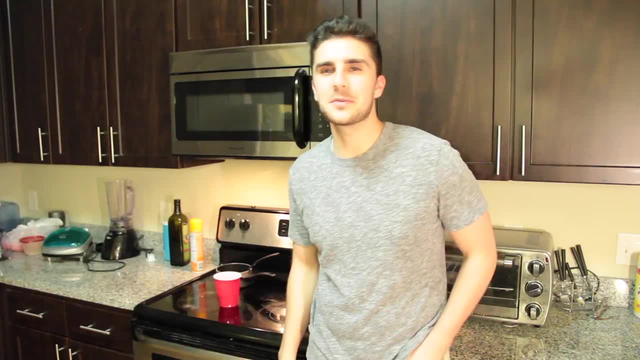 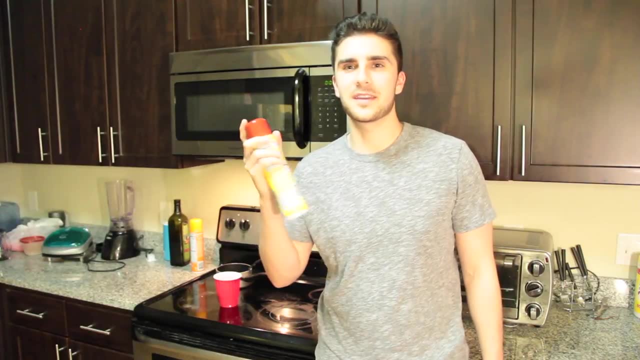 Oh, what's up guys? It's funny seeing you here. Organic chemistry is involved in everything when we're cooking in the kitchen. It's involved in the gas that heats up your stove. It's involved in the oil that gives you that non-stick performance. 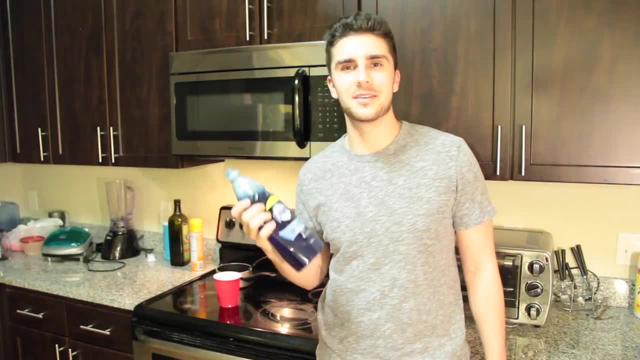 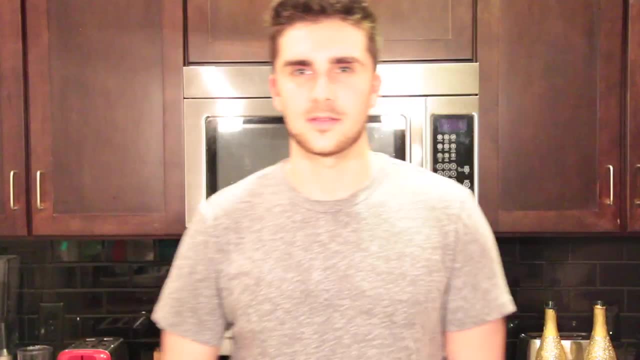 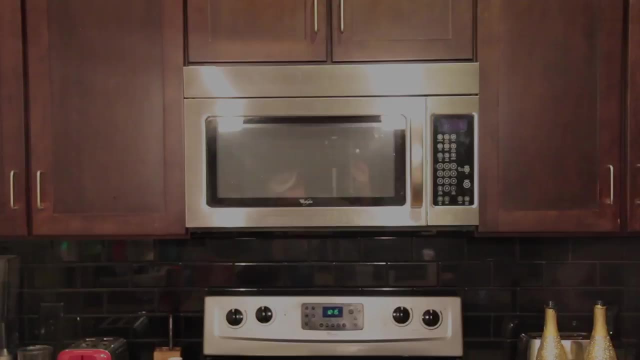 And it's involved in the soap that helps you clean those dishes after you cook a great meal. Why can you never trust atoms? Because they make up everything. Don't worry now. A simple combustion reaction is what's responsible for heating your stove to make your food. 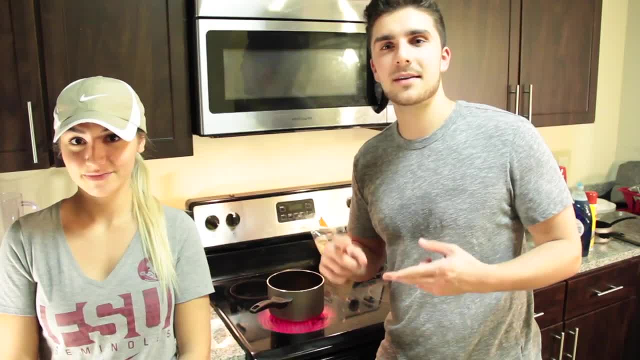 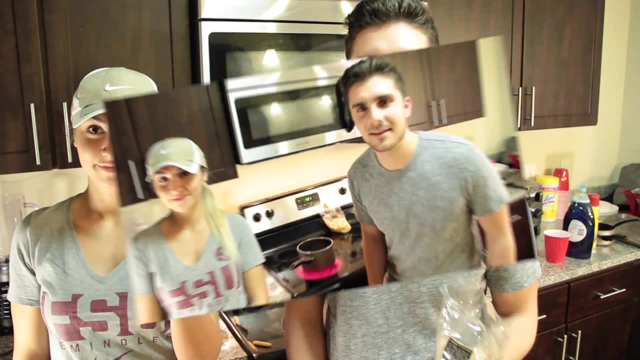 That's right. Methane and oxygen react to produce carbon dioxide, water and energy. The water and energy are what's going to be converting to electricity. That's what's going to make it piping hot. Shown here is a simple alkane, otherwise known as vegetable oils such as canola. 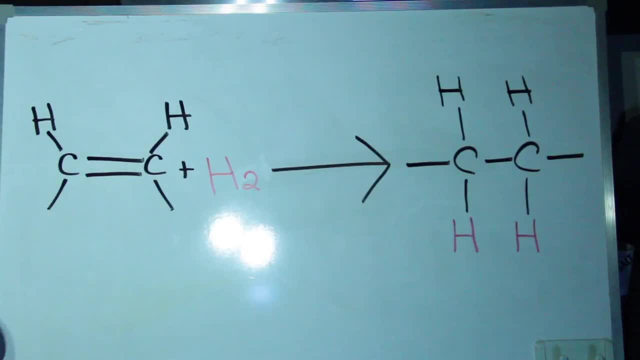 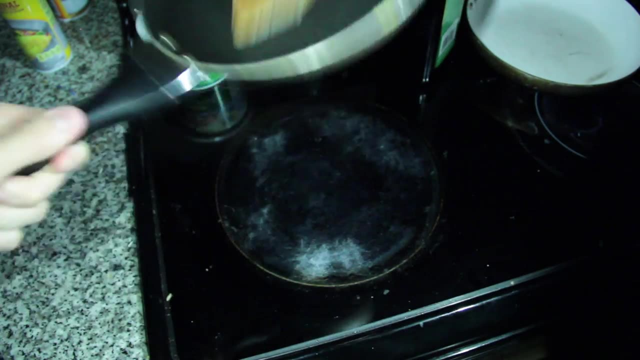 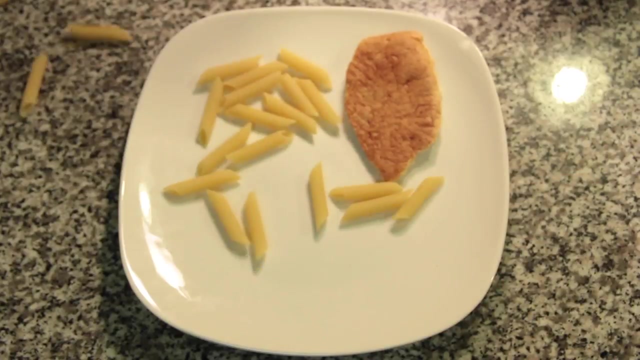 It is then hydrogenated to give you a hydrogenated alkane, Otherwise known as a hydrogenated alkane. It's also known as various cooking fats like margarine. Wow, what a nutritious looking meal. Now it's time to clean up. 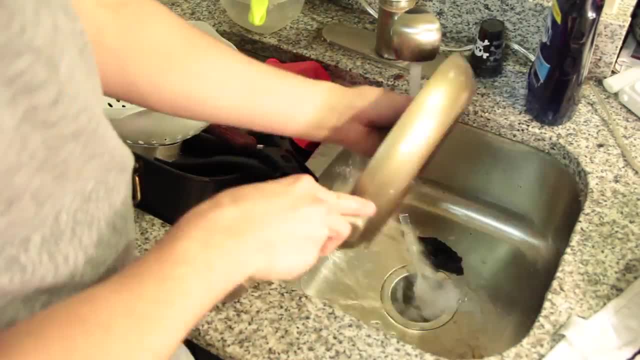 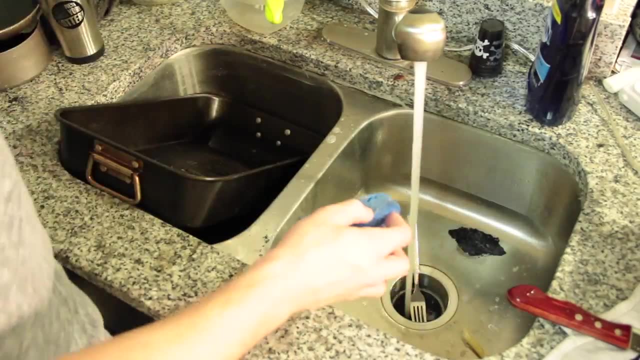 Soap is made up of molecules with hydrophobic and hydrophilic ends. One end of soap molecules love water. the other end of soap molecules hate water. The hydrophobic ends of soap molecules attach to the oil, making it from the surface, leaving your pots and pans spotless. 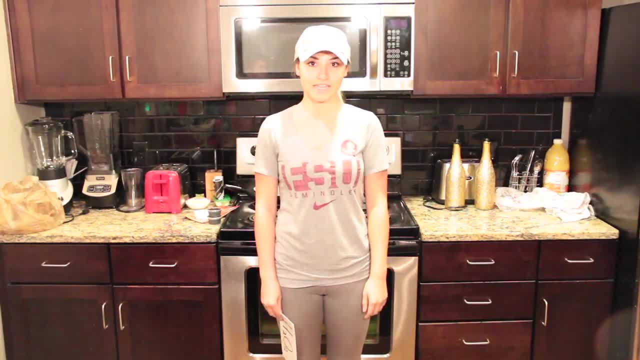 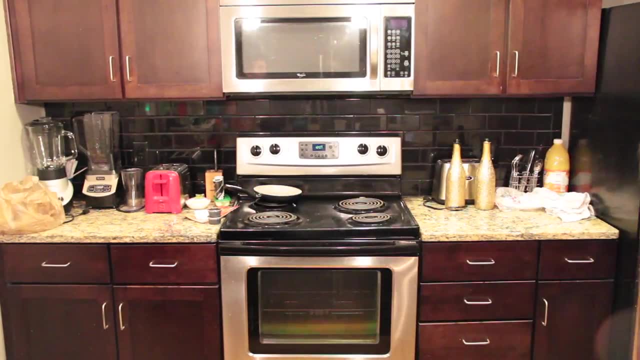 Two chemists walk into a bar. One says I'll have an H2O, The other one says I'll have an H2O2.. Then he died. The more you know. Alright, bye, mom. Thank you guys for watching our video. 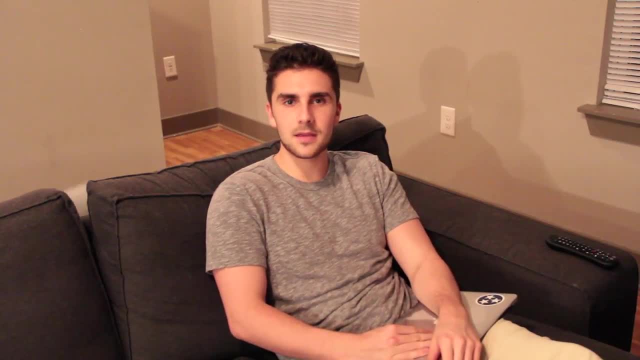 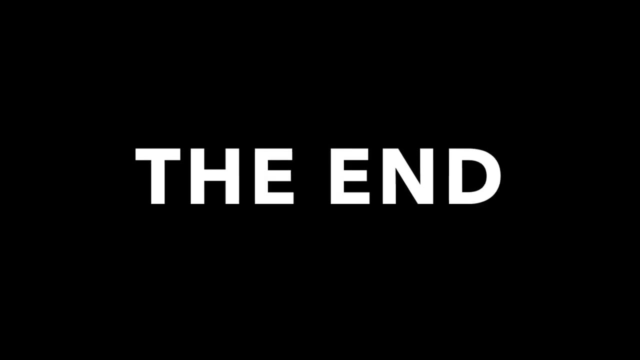 Organic chemistry is really hard. I'm Cameron Tate And I'm Katrina Miller, And this has been The More You Know. Subtitles by the Amaraorg community.